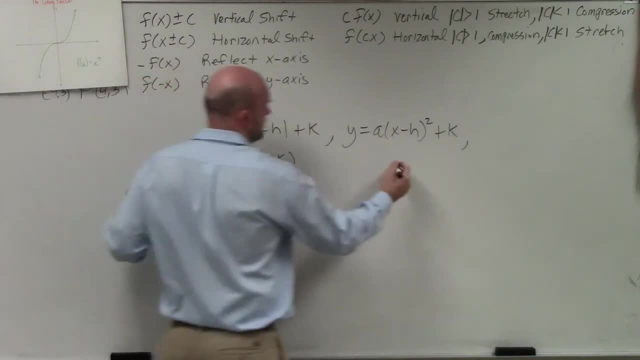 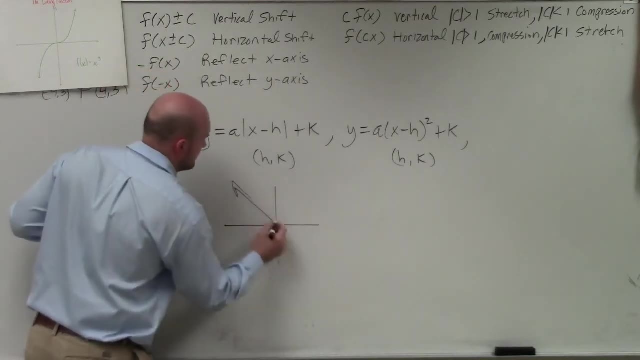 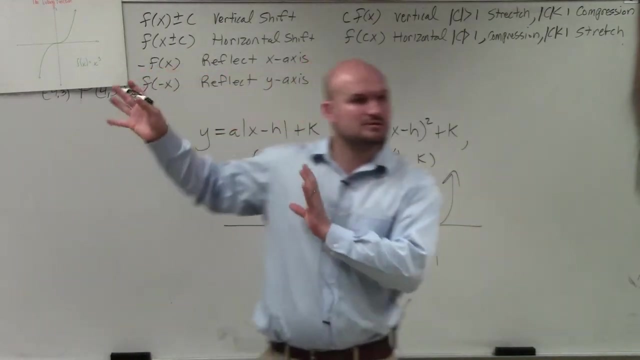 our minimum point was H comma K, H comma K, right? And if you're graphing them, these graphs look very, Very similar to each other, correct? When you guys are doing your little thing that we did last class period, they almost said they. Actually they do have the exact same. 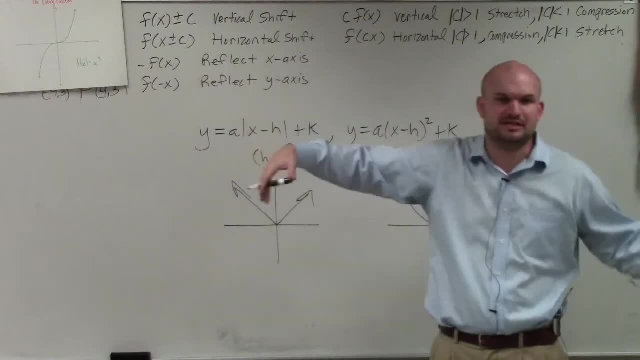 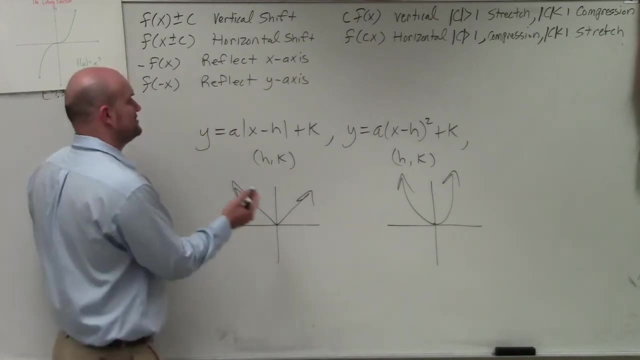 answer for everything we did last class period: The minimum, the maximum, the increasing, decreasing and behavior and all that kind of stuff. So they look very similar to each other And remember that a lot of students always kind of got confused because they're 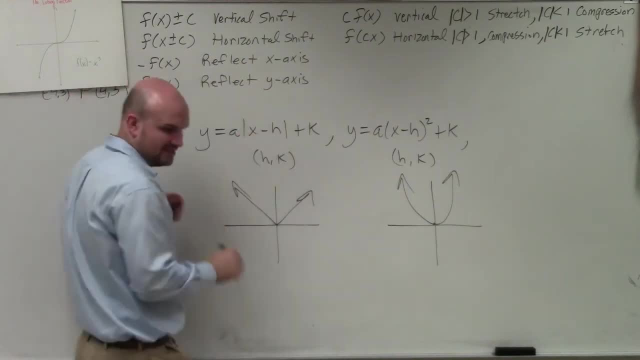 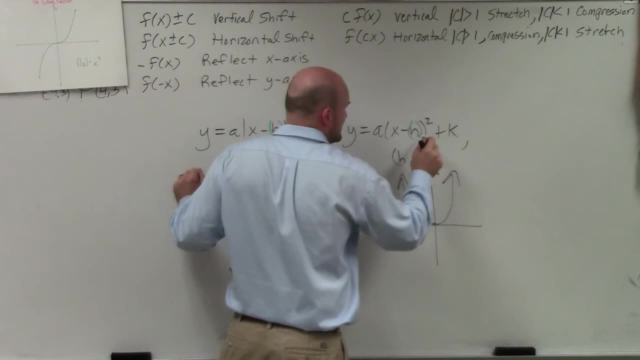 like: oh, when it was like. you know, Remember, this can really technically be written like this: X minus H in parentheses. X minus H in parentheses, because what gets everybody so confused is when I have, you know, X minus 1 squared, everybody wants to say that the vertex is negative 1, and let's 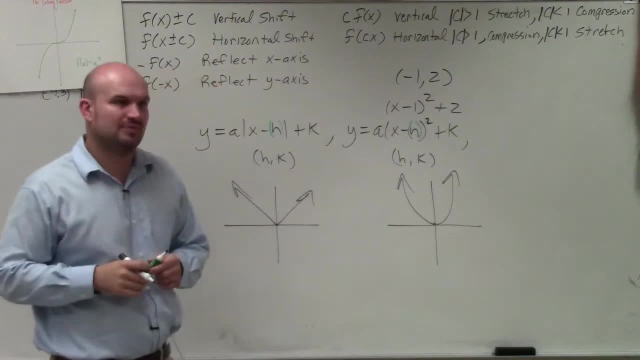 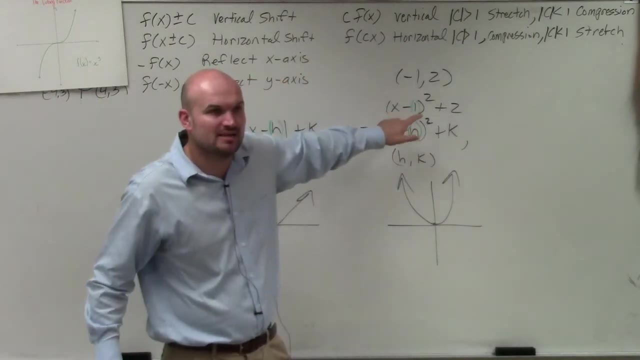 say plus 2.. Everybody wants to say it's negative 1 plus 2, but remember that value. you can think of that as inside parentheses. What is that value of 1? inside the parentheses One, because it's X minus the value of H. That's a lot easier Because when we got the, There's a liquid component, Yeah, And we case value for that, What? That's a lot easier. This part of it is really not so much, because, by the way, people don't still buy things that are chase-h. 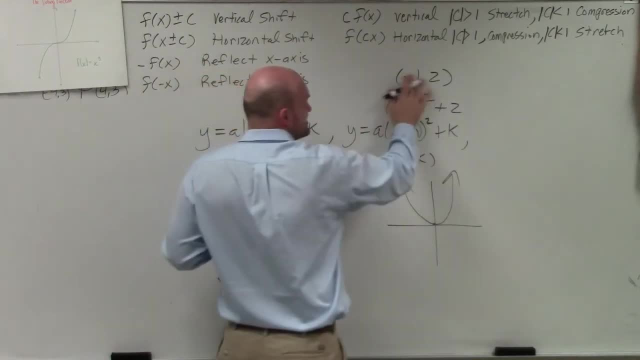 Okay, that's a lot easier. Who did you say it? You say it's a question. The question is Question 1, x minus h minus h in parentheses. The value of h in this case is 1.. So the vertex is 1 comma, 1 half. 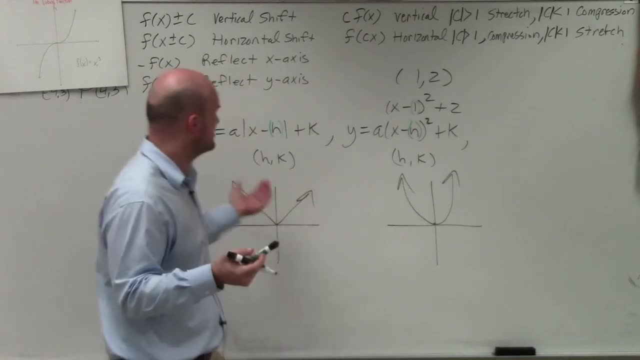 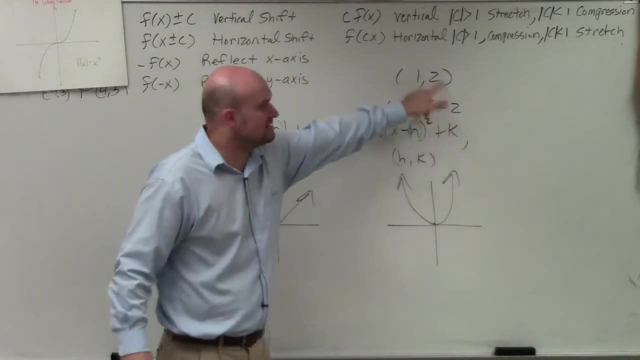 So the easy way to just kind of think about that is if you just say it's always the opposite. You can always just think of inside the function as the opposite, whereas k is always the same value of what it is. Again, think about it this way: 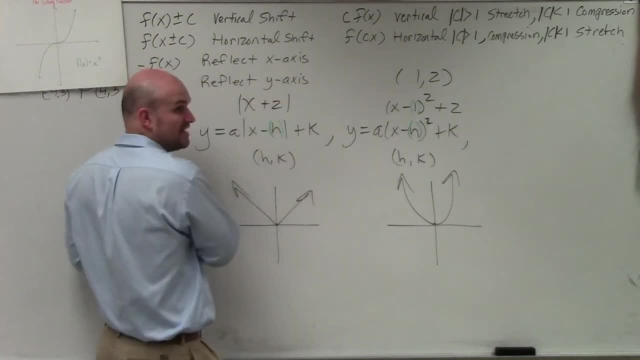 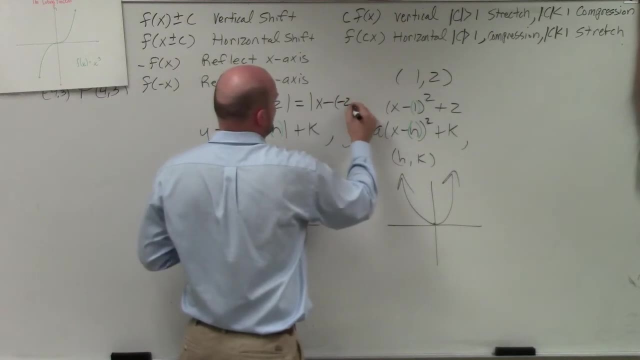 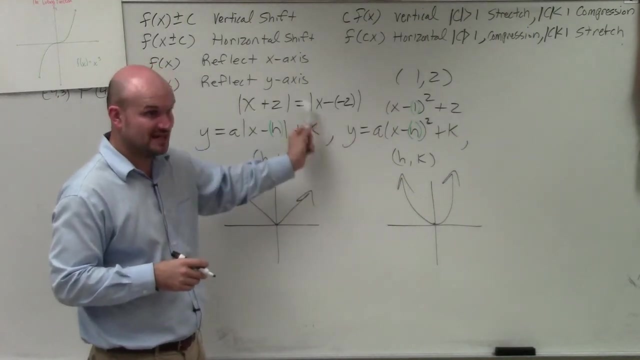 x plus 2.. That h is equal to negative 2.. Why? Because x minus a negative 2 is the same way to say x plus 2.. That's x minus h. Would you guys agree with me? That's x minus h. 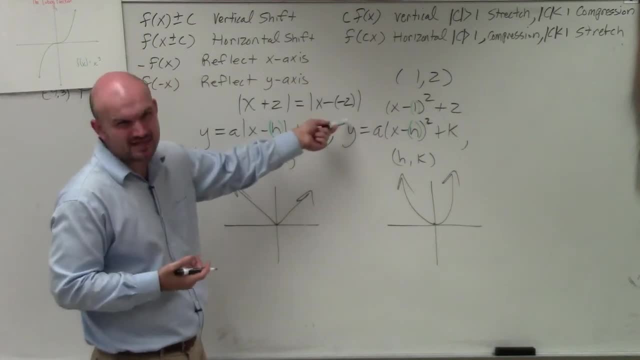 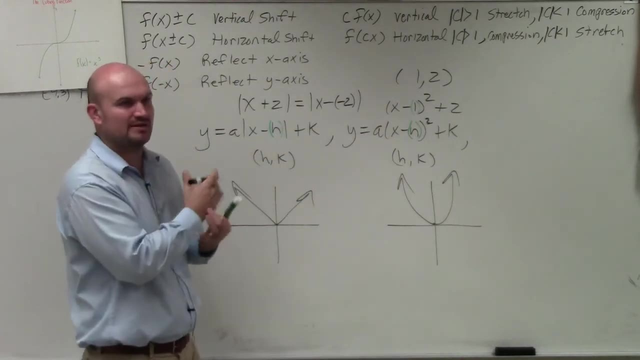 x minus h, where h is negative 2.. But we don't write things x minus a negative number. We simplify that to x plus h. That's why it's always the opposite way that it's written, because it's being simplified in our format.